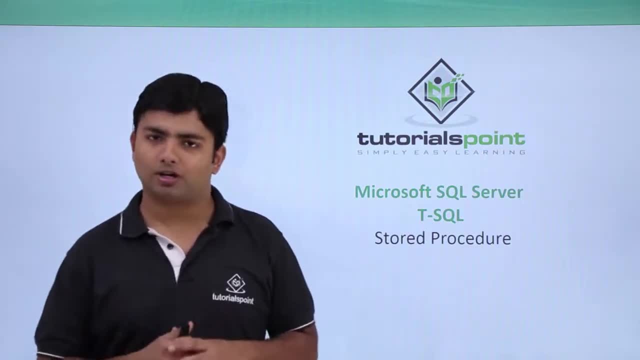 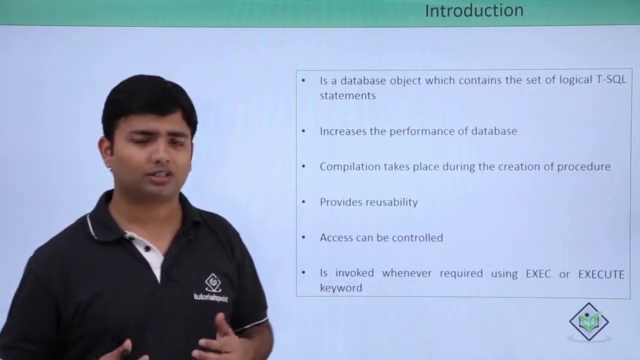 So that, whenever required, we can call them up. And one of the way of doing that is by stored procedure, As stored procedure is one of the database object which actually stores the transact, a logical transact SQL block. When I say logical, that means it must be doing some particular task. 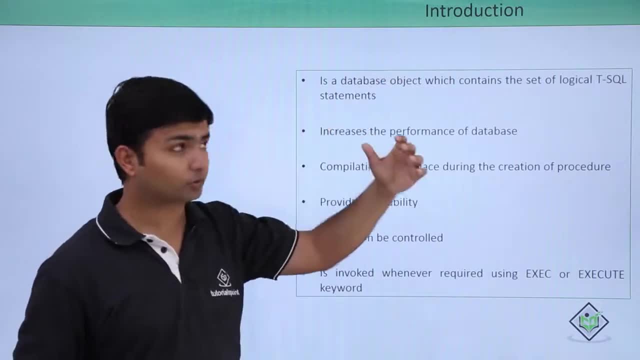 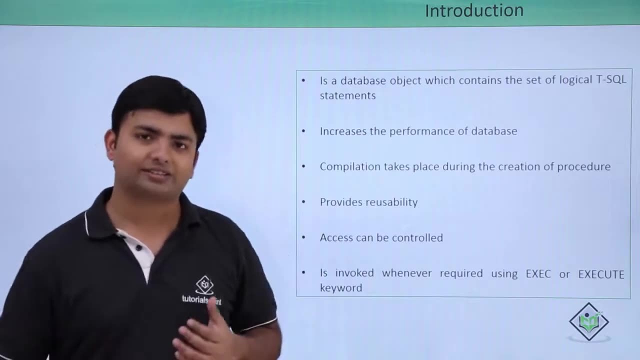 So that is what we can do, by using the stored procedure. It is a database object which contains a set of logical TSQL statements. It also increases the performance of the database, So I am going to show you how to do that. Basically, whenever we were executing the block, it was first getting compiled and then it got executed. So every time when we execute that, the compilation time is included. But when we create the stored procedure at the time we created, the compilation is done. 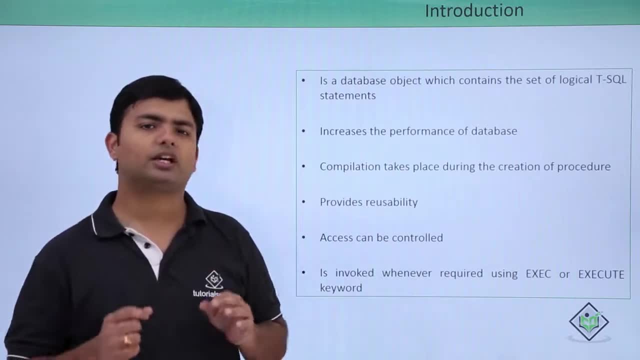 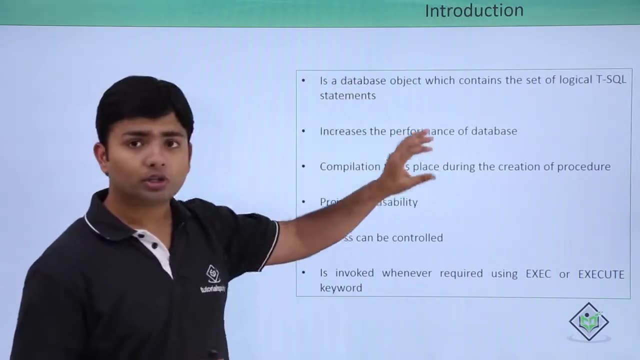 So after that, whenever we execute that, only the execution time will be elapsed As the compilation is completed, So you can see that the compilation is already done. So this is how the performance benefit will be there by the time you will be working with stored procedure. 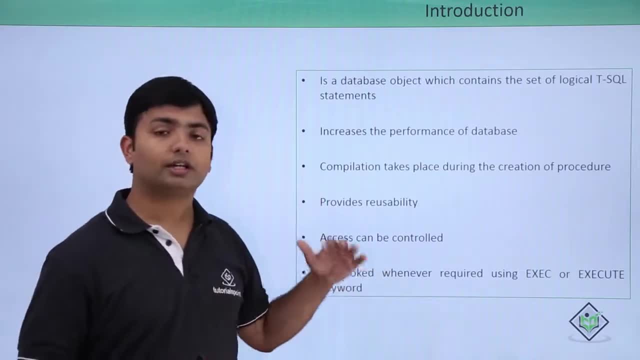 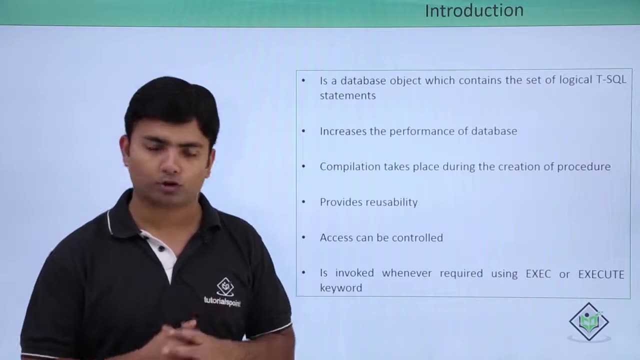 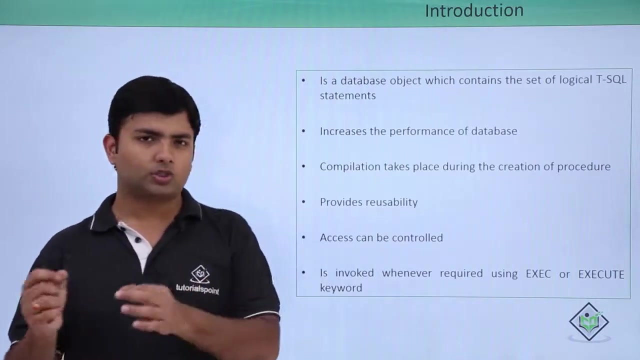 As I said earlier, it will also allow you for the reusability, as once a procedure is created, you can call it as many as times you want. The access can also be controlled, as it is a database object and for a particular audience you can grant the access of the database object as well. 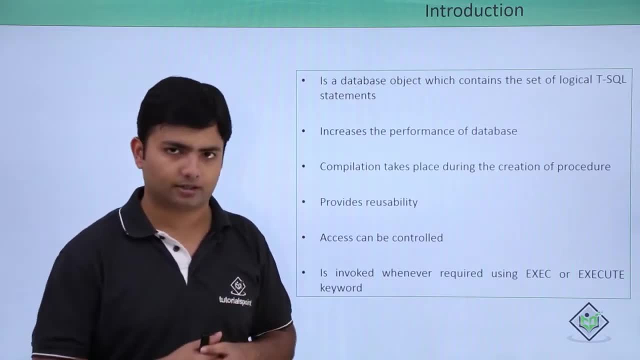 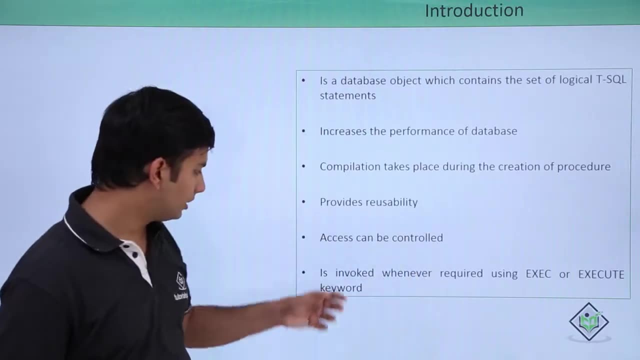 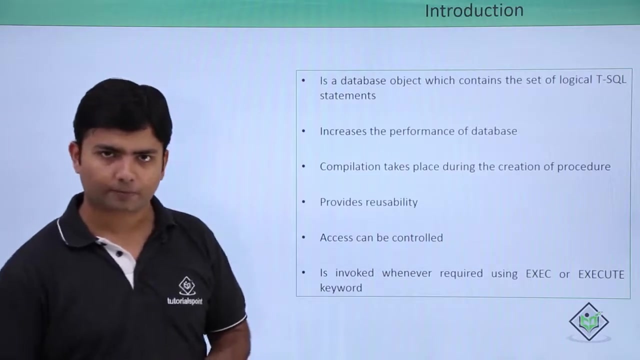 this procedure and for some particular you may not grant so it is. its access can be controlled as well and whenever you want to invoke that it is, it can be invoked directly or by using the exec or execute keyword. so, firstly, we will see how can we create the procedure using the create. 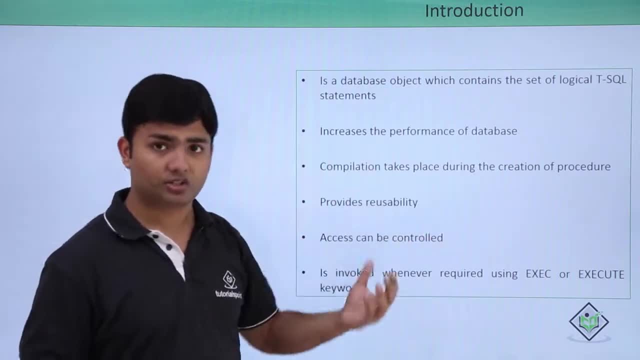 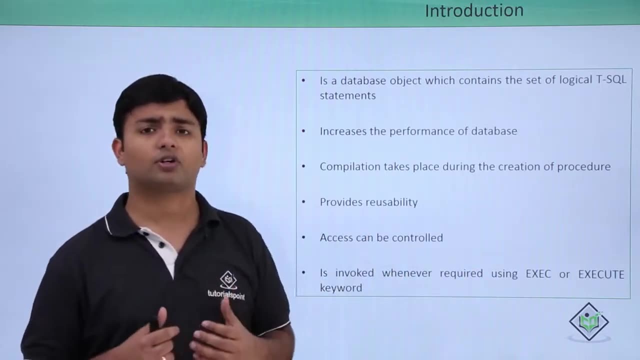 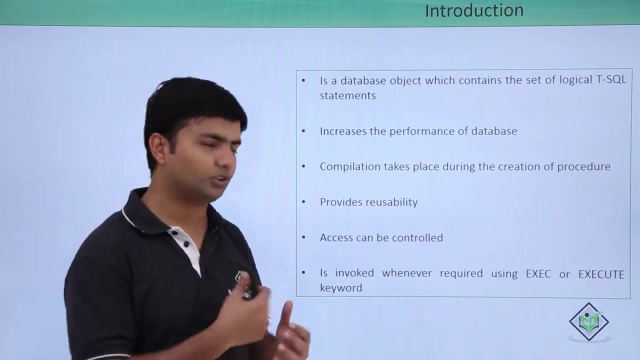 keyword again once it is done, once, once the creation is done, we will see how can we execute, and initially we will write a simple stored procedure and after we'll start writing the complex parameterized stored procedures. so let's find out practically about the stored procedures. so now, as you have already seen this particular program in the previous example of cursors, 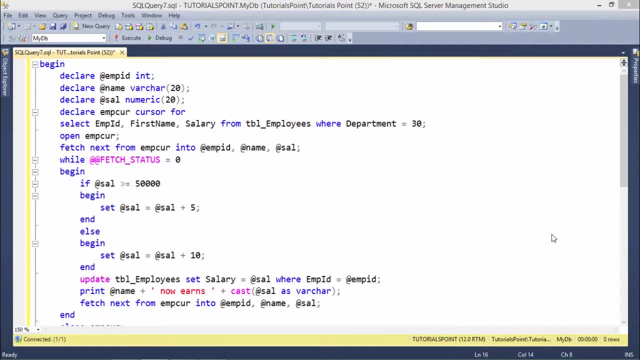 if i find it is useful enough so that i can store it permanently for the future usage, i can plan to store it as the stored procedure. now to make it stored procedure. you can use the stored procedure as the stored procedure and you can use the stored procedure. 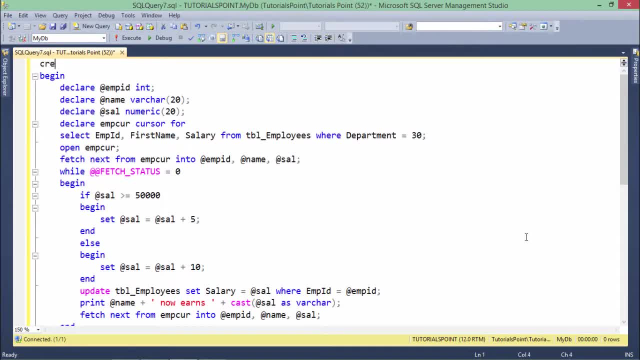 for the only thing i'll have to do in the very first line i'll just write create trock or procedure. in short, you can also write trock and then procedure name, like emp, cell increment. that's the name of procedure and then as keyword: so now this particular procedure. 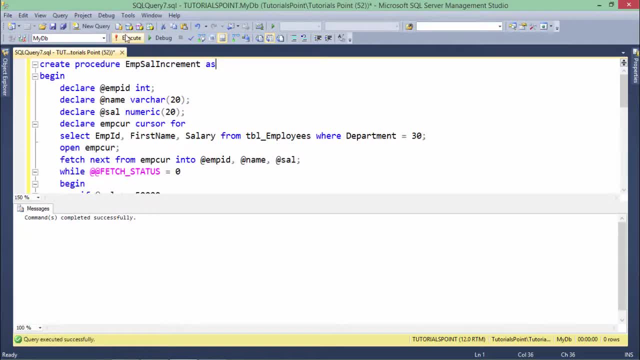 is if, when you will execute, the procedure will be created with the compilation. so every time when you will execute this emp cell increment, you will be able to create this particular procedure increment. it will just make the increment on all the employees working in department 30, but every time, in incrementing the salary of department 30 only may not be the good idea. 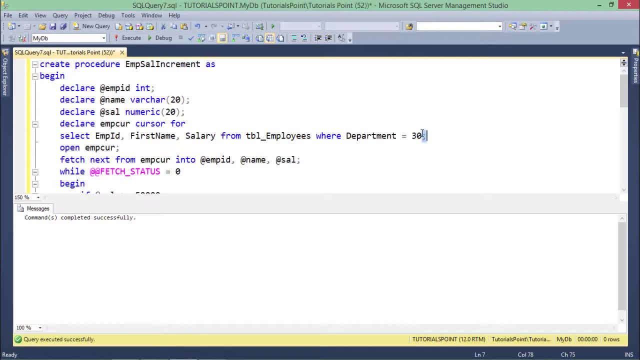 so i want to make it generalized like: whatever the department i want to increment means in whichever department i want to do the increment, i should be able to pass that at the runtime. so for doing that, what i can do, since the procedure is already created. so i will replace. 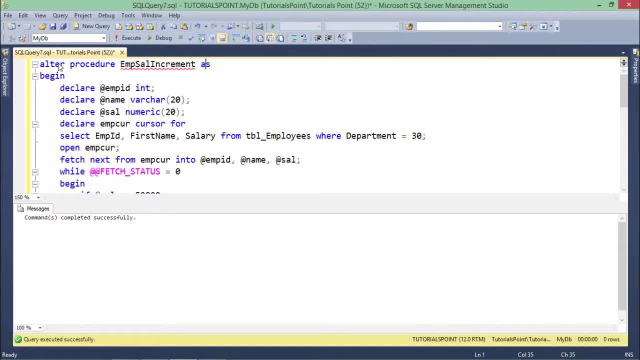 this create with the alter, since i am going to alter the structure. and now, in this emp cell increment store procedure, i will add the department as the parameter. so dept id as int and this is what. this is the parameter for the stored procedure: emp cell increment. so let's execute it. 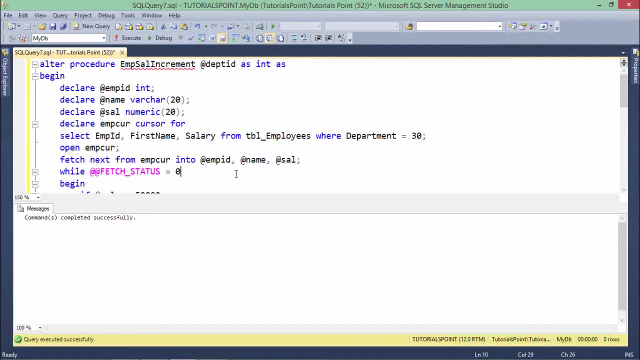 again and you see, command complete it successfully. now i will be able to call this at the runtime. and not only that, because i have add the argument here. so rather than passing 30, i will use this value right here. so every time when i will call this procedure i'll have to pass a department id, so all the searching will be done. 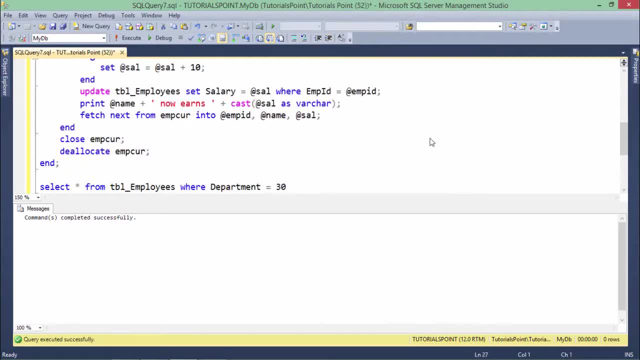 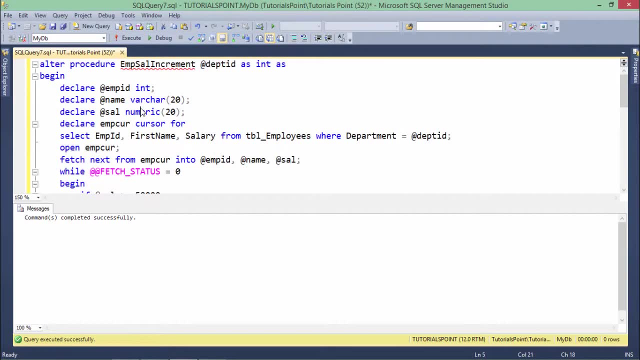 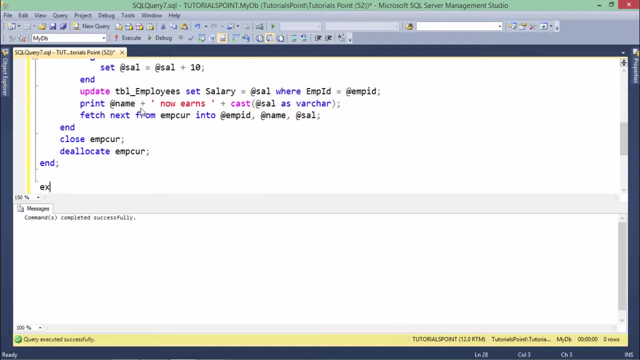 on that department employees accordingly. all right, so let's do that. let's execute it again. all right, so now it is altered. so let's now see how can we execute this stored procedure. so for executing, either i can use this execute exec or execute keyword, or after and after that, what i'll? 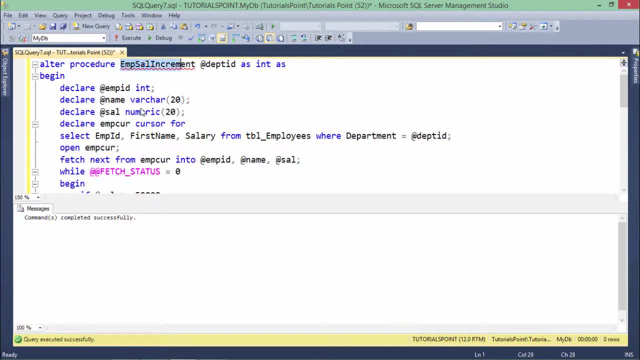 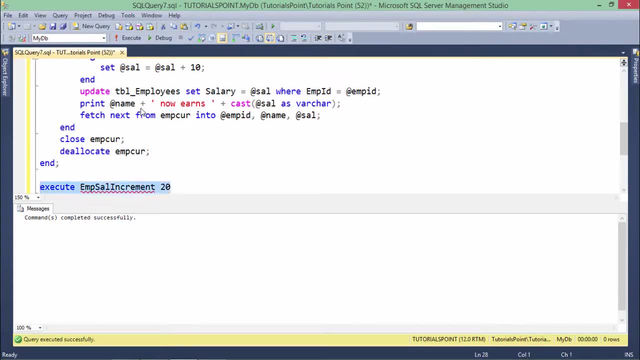 do? i'll just pass the name of this stored procedure, that is, emp cell increment, and after that i'll have to pass the department id. so as soon as i'll do that, let's execute, and you see all the employees working in that particular department. the salary got increased. 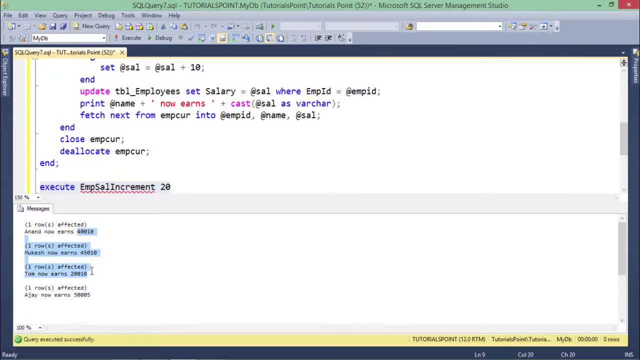 all right. so everyone who are earning less than 50 000 being salary being increment by 10, and if someone is earning greater than or equal to 50 000, the salary is increased by 5.. so this is how you can create this stored procedure and at the runtime, you can pass the parameters to make the changes. 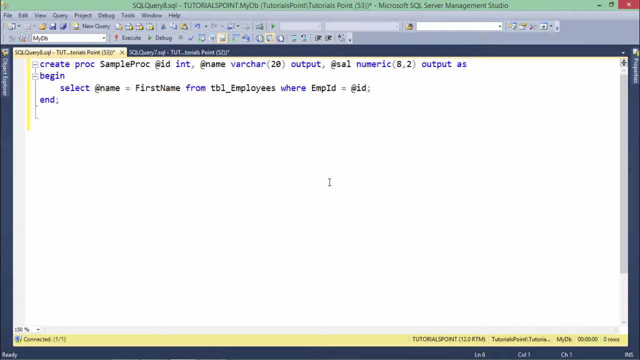 now let's have one more example of stored procedure and here what i have done. i have used two different types of parameters. like in the previous example, what i did, i passed the parameter in which, by the time of execution, i passed some value into that and, as per that value, 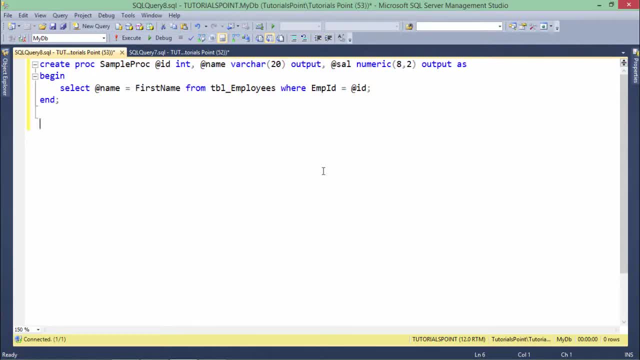 the operation got occurred. now, here i am using two different types of parameter like. the first one is the id which i have to pass when i will call this sample procedure. but apart from that, we have two more arguments, such as name and salary. but the main thing out here is these are of output types. 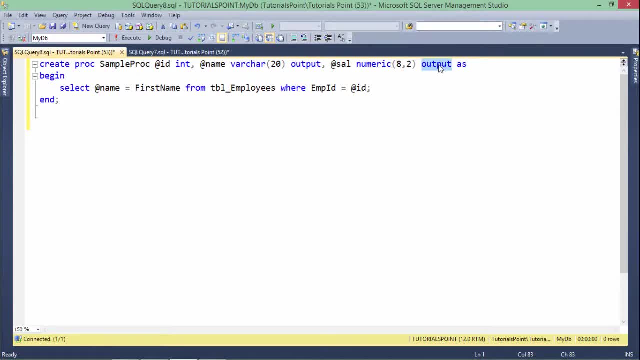 output means here for these particular parameters we actually will not pass any value by the time we will call it, but these parameter will pass some value to the calling environment means they are reversed in the direction. so far in for parameters like this we used to pass the value. 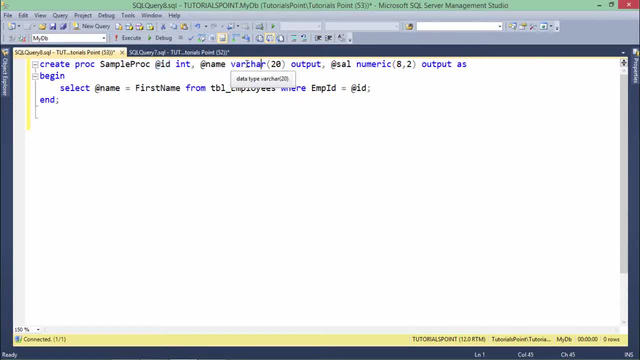 from the calling environment, but they will pass the value to the calling environment. so, for implementing, let's execute this. first, to create, now this procedure has been created and now, in order to execute that again, we should materialize the data to static". I will have to pass some variables which will be able to store the value for.